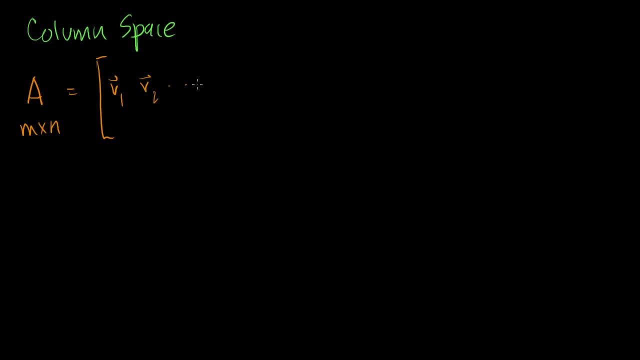 So this first one, second one, and I'll have n of them. How do I know that I have n of them? Because I have n columns And each of these column vectors are going to have how many components. So v1, v2, all the way to vn. 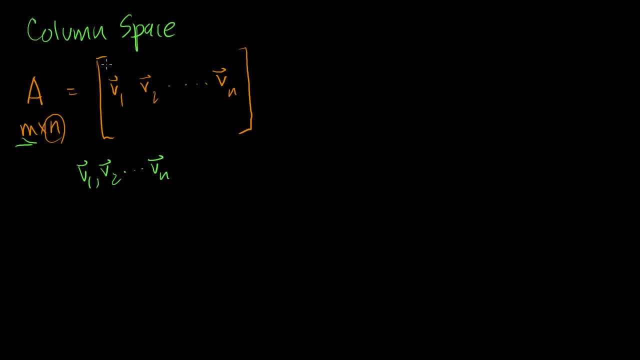 This matrix has m rows right, So each of these guys are going to have m components, So they're all members of Rm. So the column space is defined as all of the possible linear combinations of these column vectors. So the column space of A- this is my matrix- A, the column. 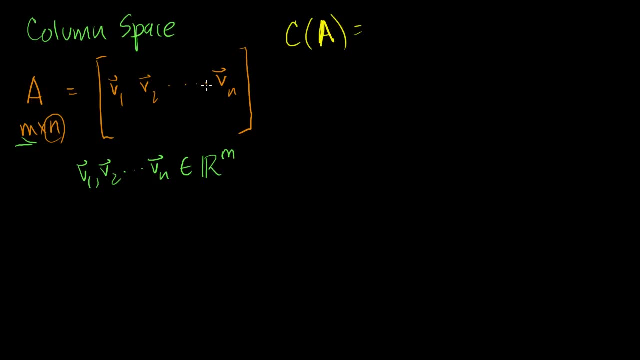 space of that is all the linear combinations of these column vectors. Well, what's all of the linear combinations of a set of vectors? It's the span. It's the span of those vectors. So it's the span of vector 1, vector 2, all the way to. 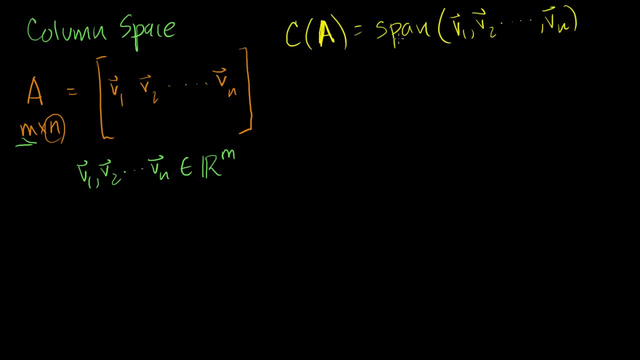 vector n, And we've done it before when we first talked about span and subspaces. but it's pretty easy to show that the span of any set of vectors is a legitimate subspace. It definitely contains the 0 vector If you multiply all of these guys by 0, which is a valid 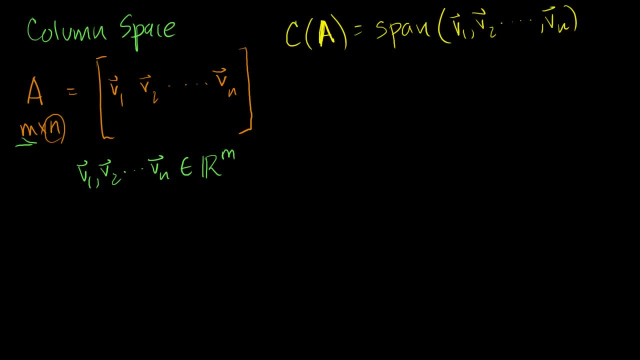 linear combination added up, you'll see that it contains the 0 vector. Let's say I have some vector A that is a member of the column space of A. That means it can be represented as some linear combination. So A is equal to c1 times vector 1 plus c2 times vector. 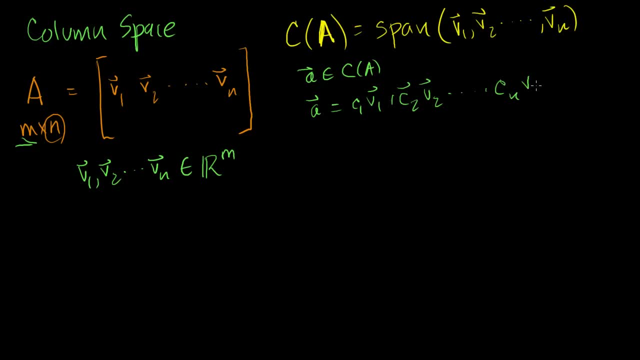 2, all the way to cn times vector n. Now the question is: is this closed? under multiplication? Is if I multiply A times some new, let me say I multiply it times some scalar s I'm just picking a random letter, so s? 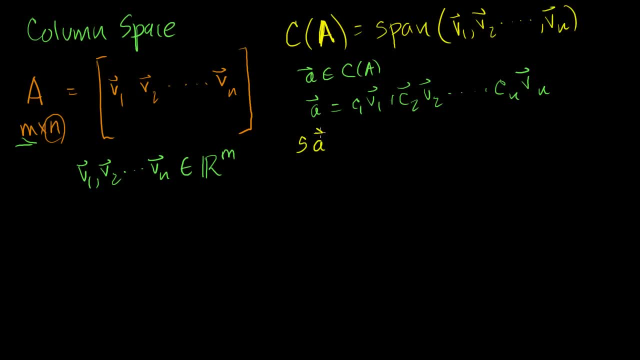 times A is this in my span. Well s times A would be equal to sc1v1 plus sc2v2, all the way to scnvn, which is once again just a linear combination of these column vectors. So this SA would clearly be a member of the. 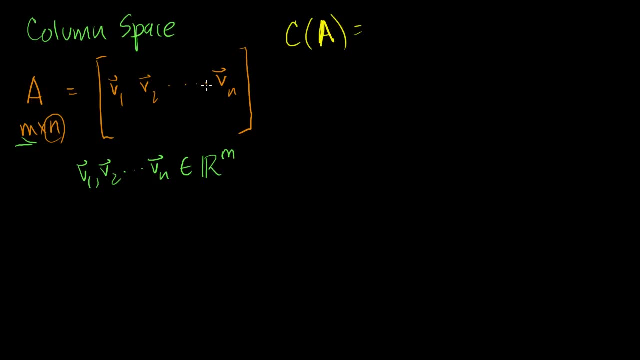 space of that is all the linear combinations of these column vectors. Well, what's all of the linear combinations of a set of vectors? It's the span. It's the span of those vectors. So it's the span of vector 1, vector 2, all the way to. 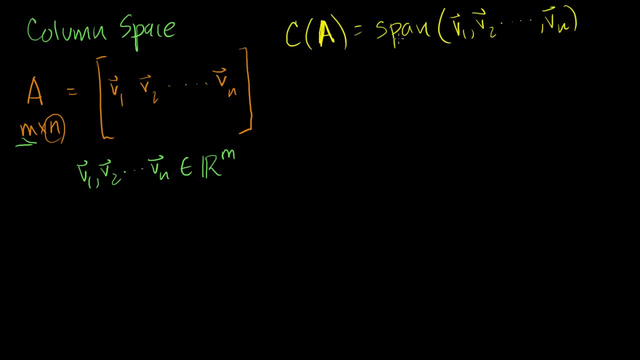 vector n, And we've done it before when we first talked about span and subspaces. but it's pretty easy to show that the span of any set of vectors is a legitimate subspace. It definitely contains the 0 vector If you multiply all of these guys by 0, which is a valid 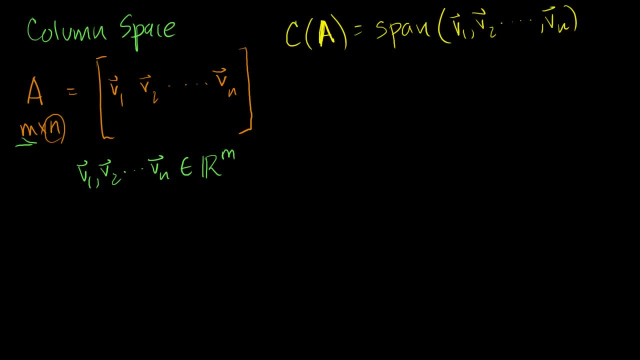 linear combination added up, you'll see that it contains the 0 vector. Let's say I have some vector A that is a member of the column space of A. That means it can be represented as some linear combination. So A is equal to c1 times vector 1 plus c2 times vector. 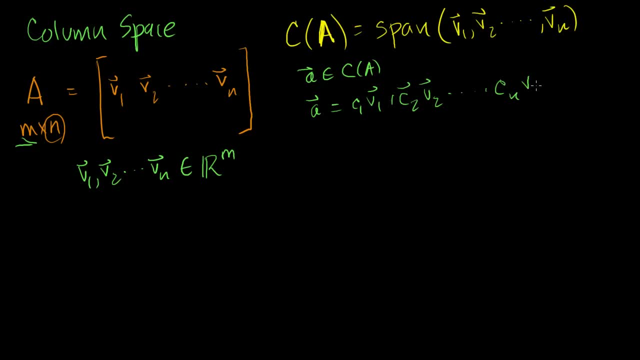 2, all the way to cn times vector n. Now the question is: is this closed? under multiplication? Is if I multiply A times some new, let me say I multiply it times some scalar s I'm just picking a random letter, so s? 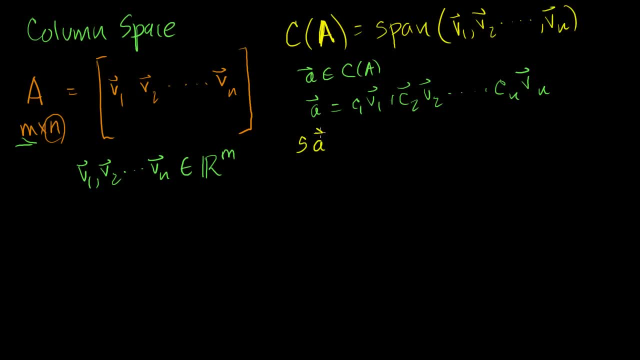 times A is this in my span. Well s times A would be equal to sc1v1 plus sc2v2, all the way to scnvn, which is once again just a linear combination of these column vectors. So this SA would clearly be a member of the. 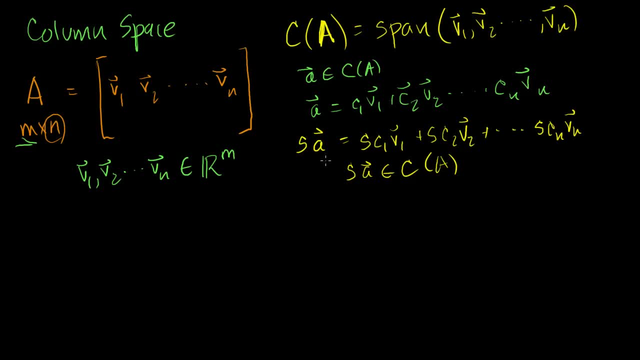 column space of A And then finally to make sure it's a valid subspace, and this actually doesn't apply just to column spaces, This applies to any span. This is actually a review Of what we've done in the past. 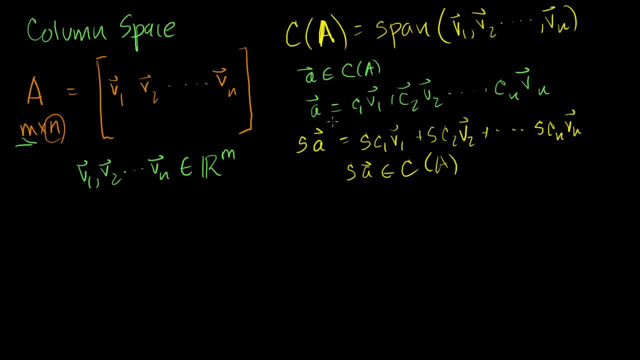 We just have to make sure it's closed under addition. So let's say A is a member of our column space. Let's say B is also a member of our column space or our span of all of these column vectors. Then B could be rewritten. as I don't know, let me say b1. 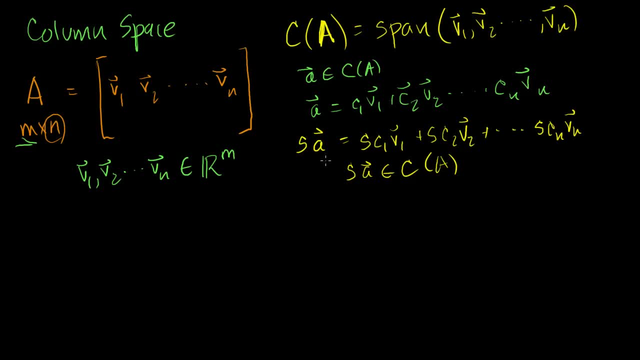 column space of A And then finally to make sure it's a valid subspace, and this actually doesn't apply just to column spaces, This applies to any span. This is actually a review Of what we've done in the past. 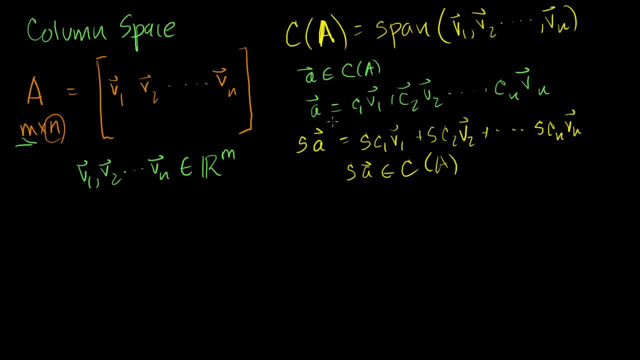 We just have to make sure it's closed under addition. So let's say A is a member of our column space. Let's say B is also a member of our column space or our span of all of these column vectors. Then B could be rewritten. as I don't know, let me say b1. 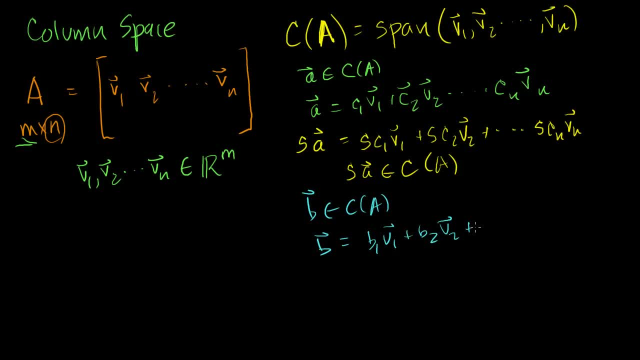 times v1 plus b2 times v2, all the way to bn times vn. And my question is: is A plus B? Is A plus B? Is A plus B a member of our span, of our column space, the span of these vectors? 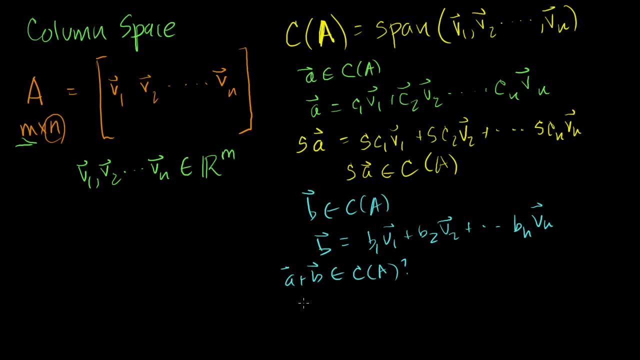 Well sure, What's A plus B? A plus B is equal to c1 plus b1 times v1, plus c2 plus b2 times v2.. I'm just literally adding this term to that term to get that term, this term to this term to get this term. 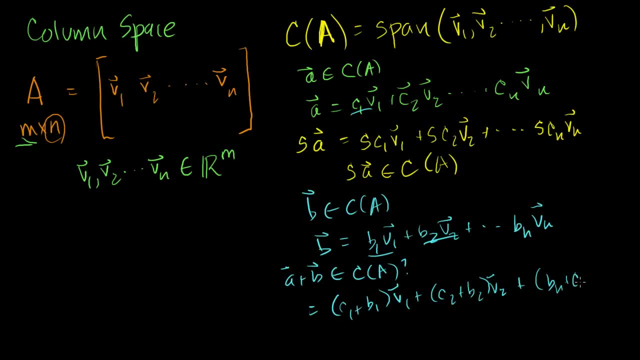 And then it goes all the way to bn plus cn times vn, which is clearly just another linear combination of these guys. So this guy is definitely within the span, So the span of and this what I just did. it doesn't have to. 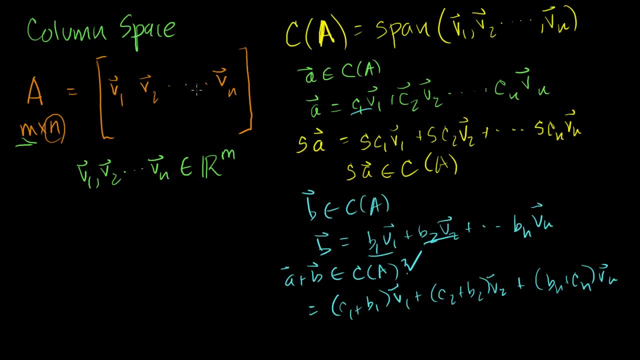 be unique to a matrix. I mean, a matrix is just, really just a way of writing a set of column vectors, So this applies to any span. So this is clearly a valid subspace. so the column space of A is clearly a valid subspace. 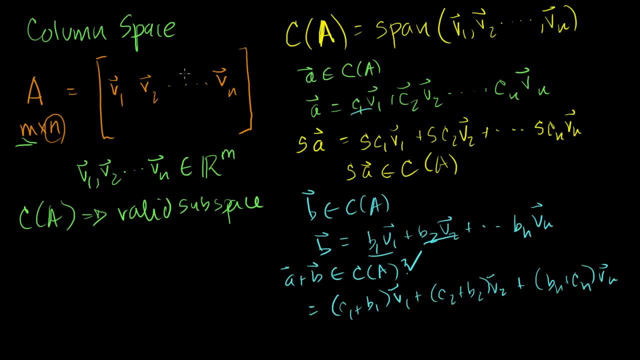 Now let's think about other ways we can interpret this notion of a column space. Let's think about it in terms of the expression: Let me get a good color If I were to multiply my. let's think about this. Let's think about the set of all the values of if I take 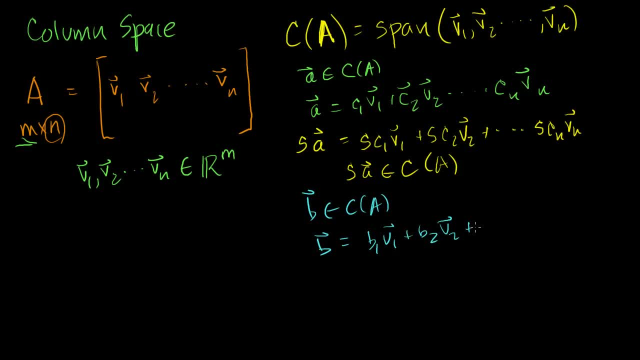 times v1 plus b2 times v2, all the way to bn times vn. And my question is: is A plus B? Is A plus B? Is A plus B a member of our span, of our column space, the span of these vectors? 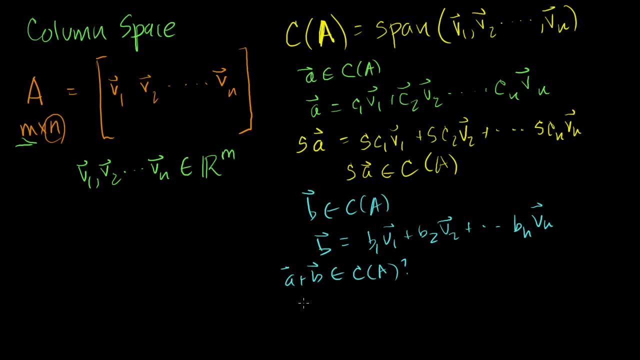 Well sure, What's A plus B? A plus B is equal to c1 plus b1 times v1, plus c2 plus b2 times v2.. I'm just literally adding this term to that term to get that term, this term to this term to get this term. 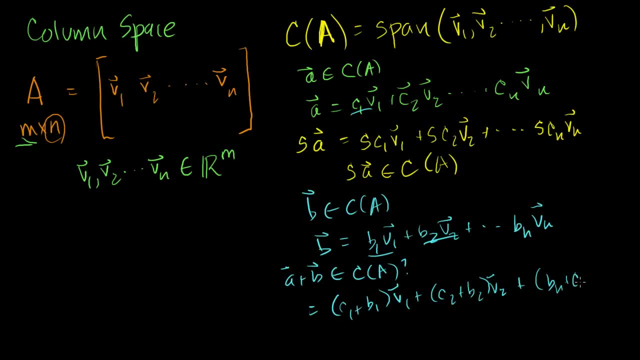 And then it goes all the way to bn plus cn times vn, which is clearly just another linear combination of these guys. So this guy is definitely within the span, So the span of and this what I just did. it doesn't have to. 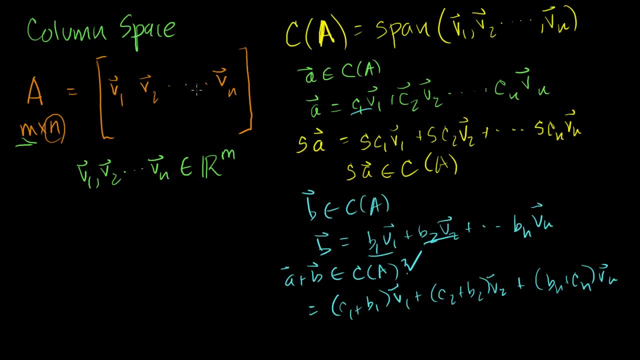 be unique to a matrix. I mean, a matrix is just, really just a way of writing a set of column vectors, So this applies to any span. So this is clearly a valid subspace. so the column space of A is clearly a valid subspace. 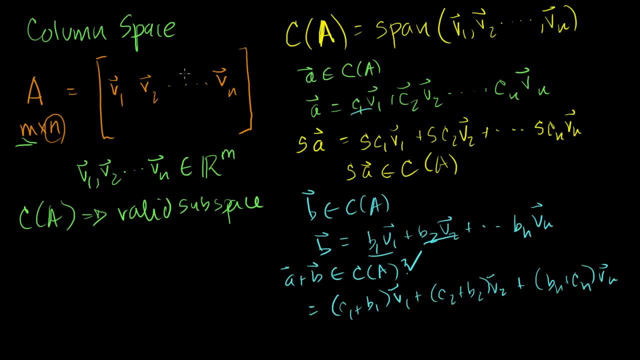 Now let's think about other ways we can interpret this notion of a column space. Let's think about it in terms of the expression: Let me get a good color If I were to multiply my. let's think about this. Let's think about the set of all the values of if I take 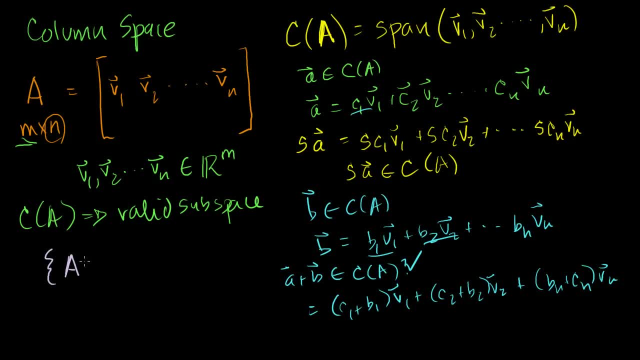 my m by n, matrix A, and I multiply it by any vector, x. where x has to be a member of Rn, It has have n components in order for this multiplication to be well-defined. So x has to be a member of Rn. 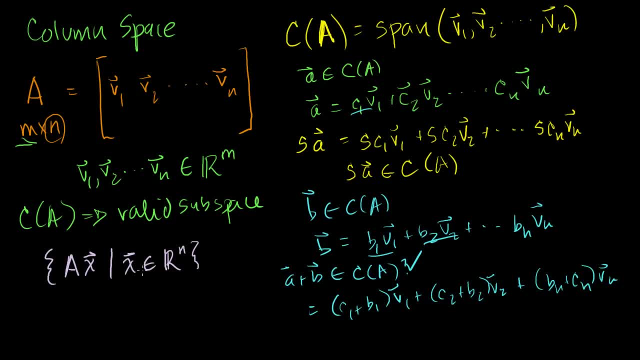 Let's think about what this means. This is the set. This says: look, I can take any member and n component vector and multiply it by A, and I care about all of the possible products that this could equal. All the They. 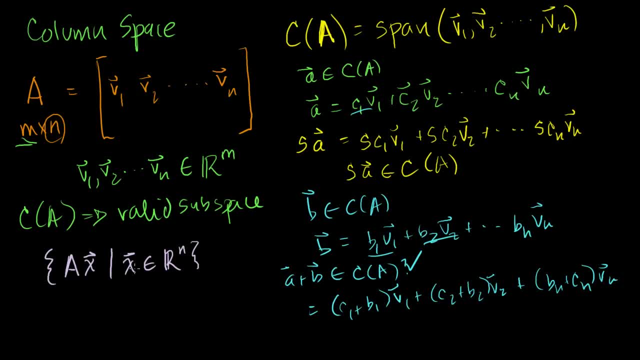 possible values of AX. when I can pick and choose any possible X from Rn, Let's think about what that means: AX, if I write A like that and if I write X like this. Let me write it a little bit better. 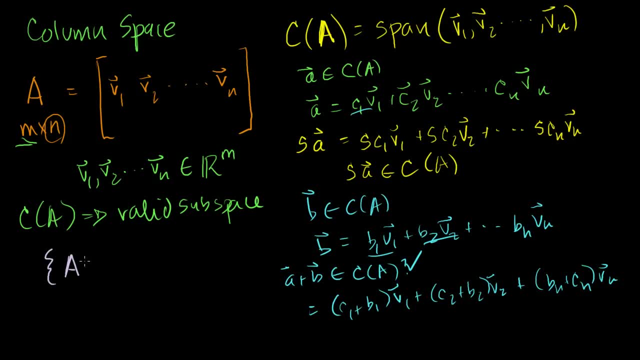 my m by n, matrix A, and I multiply it by any vector, x, where x is a member of. remember, x has to be a member of Rn. it has to have n components in order for this multiplication to be well-defined. So x has to be a member of Rn. 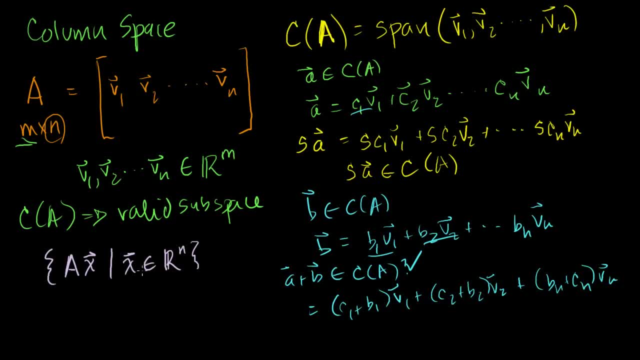 Let's think about what this means. This is the set If this says: look, I can take any member, any n component vector and multiply it by A, and I care about all of the possible products that this could equal all the. 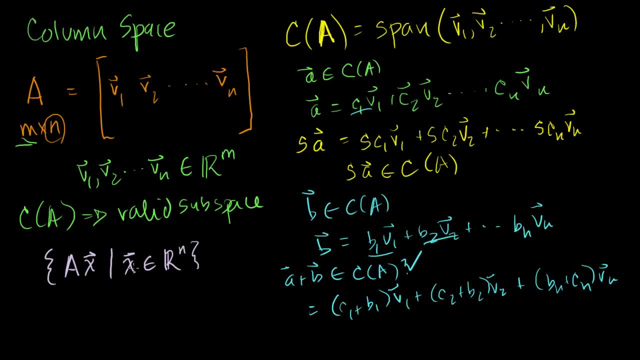 possible values of Ax. when I can pick and choose any possible x from Rn, Let's think about what that means. Ax, if I write a like that and if I write x like this, let me write it a little bit better. 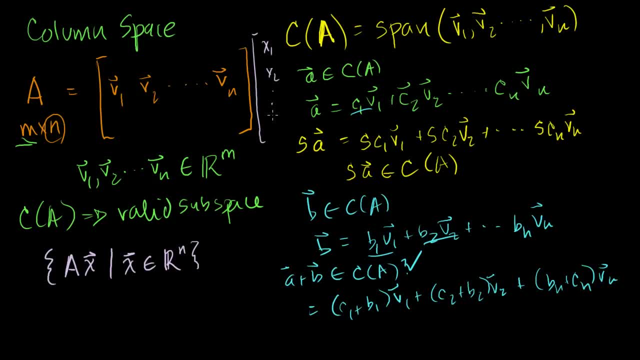 Let me write x like this: x1,, x2, all the way to xn. What is Ax? Well, Ax could be rewritten as x1,, and we've seen this before. Ax is equal to x1 times v1 plus x2 times v2, all the way. 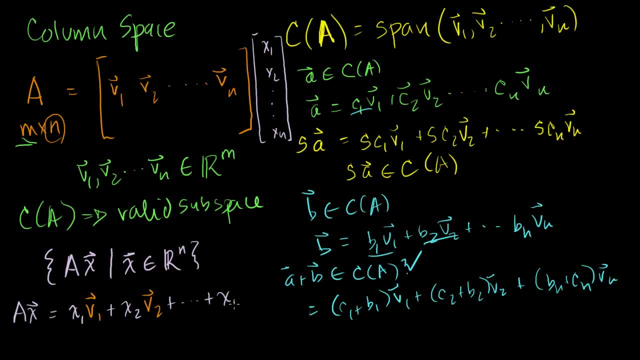 to plus xn times vn. We've seen this multiple times. This comes out of our definition of matrix vector products. Now, if Ax is equal to this, If Ax is equal to this- and I'm essentially saying that I can pick any vector- x and Rn- I'm saying that I can pick all. 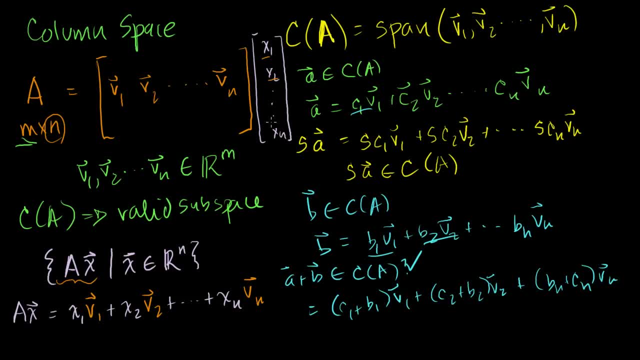 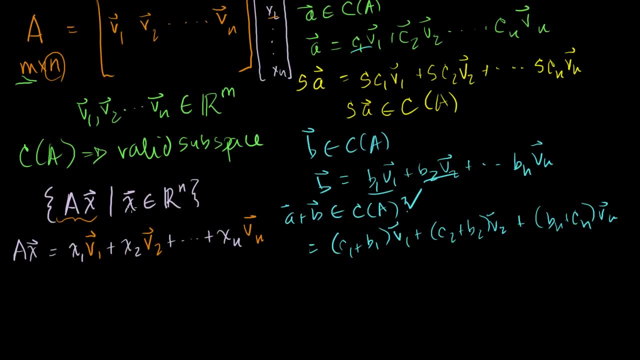 possible values of the entries here, all possible real values and all possible combinations of them. So what is this equal to? What is the set of all possible? So I could rewrite this statement here as the set of all possible: x1, v1 plus x2, v2, all the way to xn, vn. 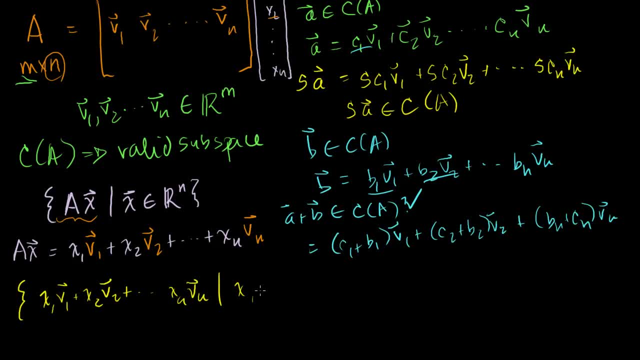 Where x1,, x2, all the way to xn- are a member of the real numbers. That's all I'm saying here. This statement is the equivalent of this When I say that the vector x can be any member of Rn. I'm. 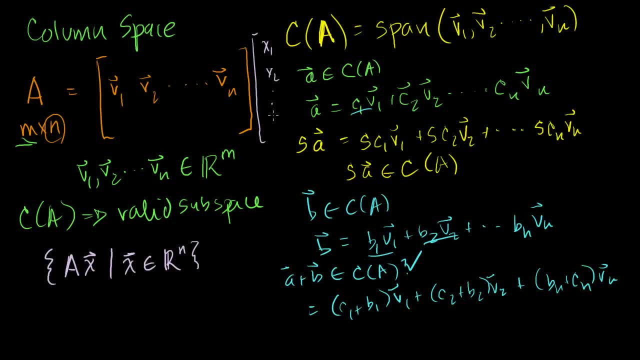 Let me write X like this: X1, X2, all the way to Xn. What is AX? Well, AX could be rewritten as X1,- and we've seen this before- AX is equal to X1 times V1 plus X2 times V2, all the way. 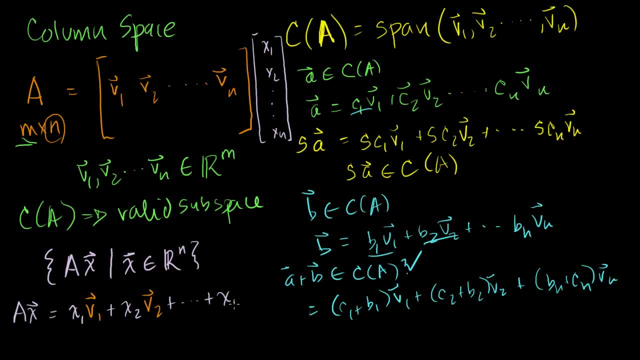 to plus Xn times Vn. We've seen this multiple times. This comes out of our definition of matrix vector products. Now, if AX is equal to this, If AX is equal to this- and I'm essentially saying that I can pick any vector- X and Rn- I'm saying that I can pick all. 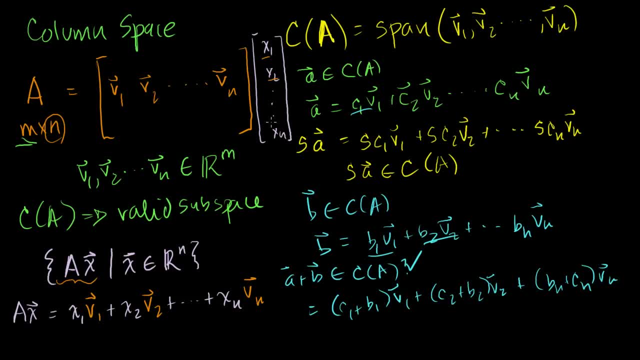 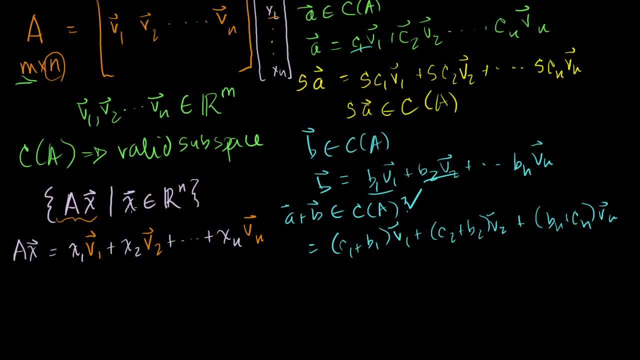 possible values of the entries here, all possible real values and all possible combinations of them. So what is this equal to? What is the set of all possible? So I could rewrite this statement here as the set of all possible: X1, V1 plus X2, V2, all the way to Xn, Vn. 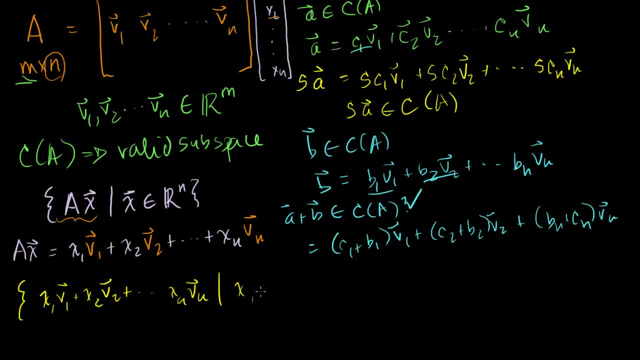 Where X1,, X2, all the way to Xn are a member of the real numbers. That's all I'm saying here. This statement is the equivalent of this When I say that the vector X can be any member of Rn. I'm. 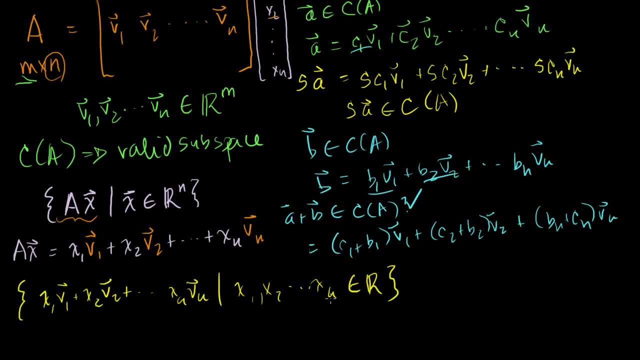 saying that its components can be any members of the real numbers. So if I just take the set of all of the, essentially the combinations of these column vectors, where they're real numbers, where their coefficients are members of the real numbers, What am I doing? 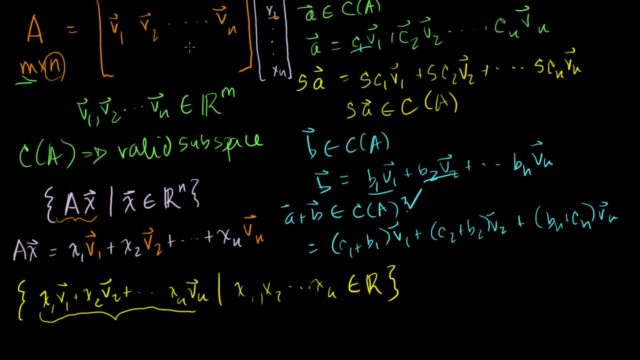 This is all the possible linear combinations of the column vectors of A. So this is equal to the span of V1, V2, all the way to Vn, which is the same, exact same thing as the column space of A. So the column space of A. you could say: hey, what are all? 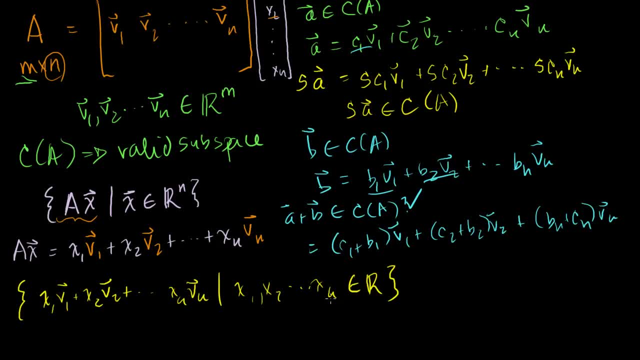 saying that its components can be any members of the real numbers. So if I just take the set of all of the, essentially the combinations of these column vectors, where they're real numbers, where their coefficients are members of the real numbers, What am I doing? 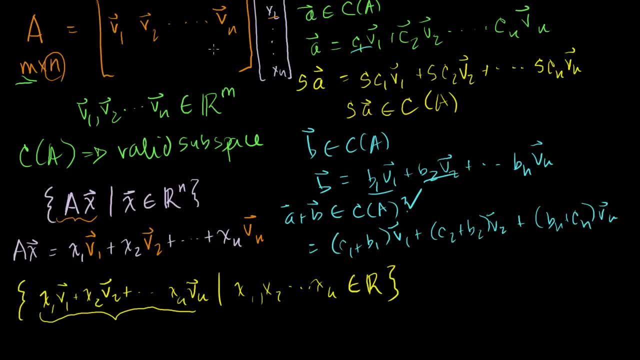 This is all the possible linear combinations of the column vectors of A. So this is equal to the span of v1, v2, all the way to vn, which is the same, exact same thing as the column space of A. So the column space of A. you could say: hey, what are all? 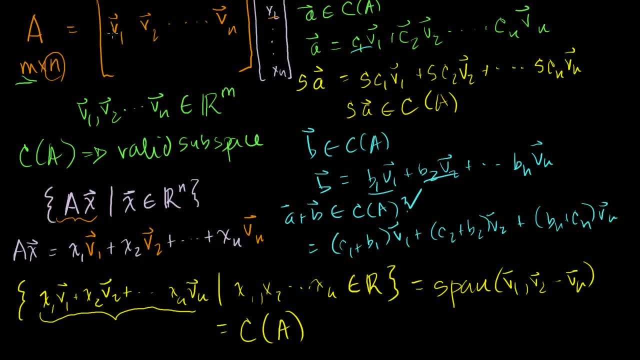 the possible vectors or the set of all vectors I can create by taking linear combinations of these guys or the span of these guys, Or you can view it as what are all of the possible values that Ax can take on if x is a member of Rn. 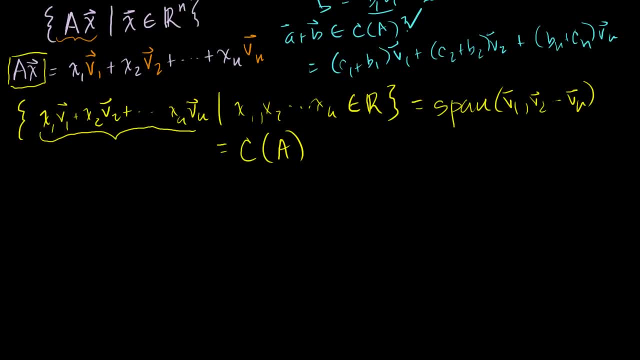 So let's think about it this way. Let's say that I were to tell you that I need to solve the equation. Ax is equal to, let me say: well, the convention is to write a b there, but let me put a special b there. 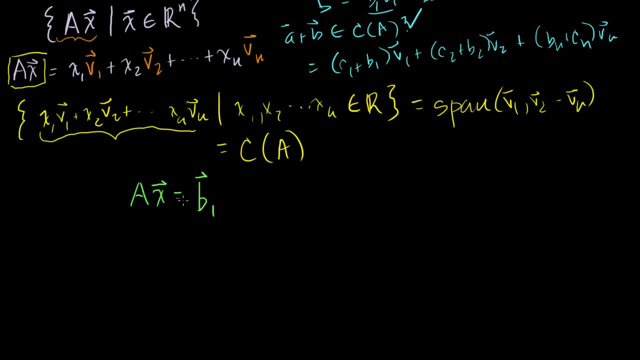 Let me put b1.. Let's say that I need to solve this equation. Ax is equal to b1.. And then I were to tell you, let's say that I were to figure out the column space of A and I say b1 is not a member. 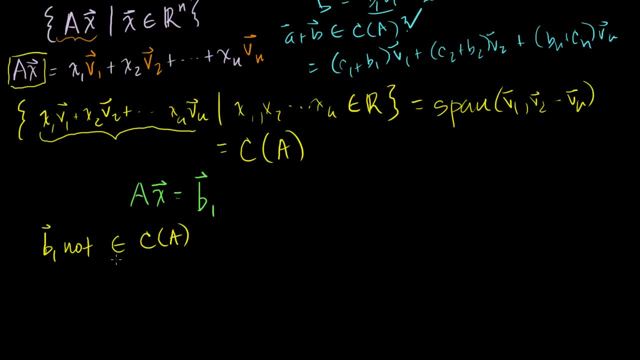 of the column space of A. Then what does that tell me? That tells me that this right here can never take on the value b1, right, Because all of the values that this can take on is the column space of A. So if b1 is not in this, it means that this can. 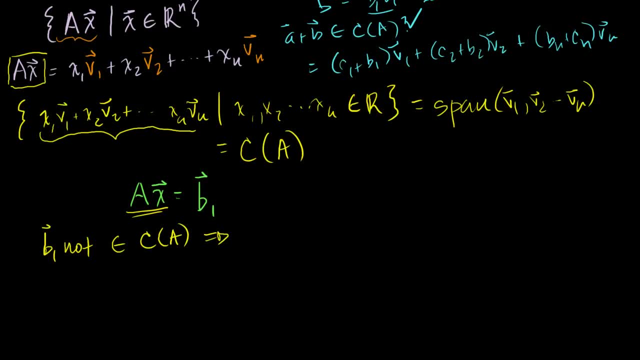 not take on the value of b1.. So this would imply that this equation we're trying to set up, Ax is equal to b1, has no solution. If it had a solution, if it had some solution. so let's say that Ax equals b2, has at least one solution. 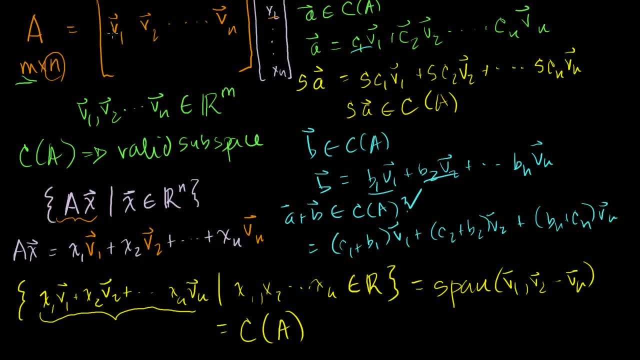 the possible vectors or the set of all vectors I can create by taking linear combinations of these guys or the span of these guys, Or you can view it as what are all of the possible values that Ax can take on if X is a member of Rn. 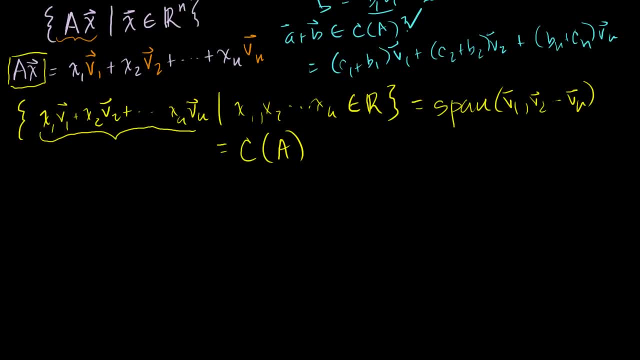 So let's think about it this way. Let's say that I were to tell you that I need to solve the equation. Ax is equal to: let me say: well, the convention is to write a B there, but let me put a special B there. 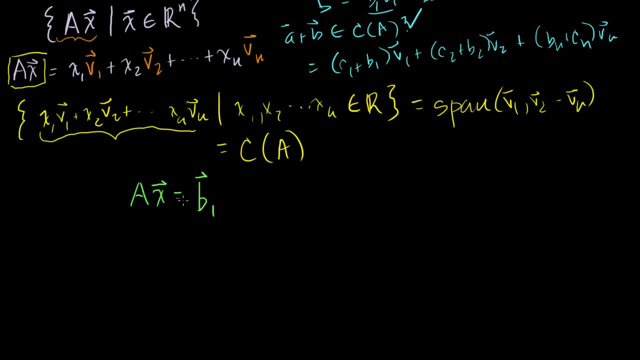 Let me put B1.. Let's say that I need to solve this equation. Ax is equal to B1. And then I were to tell you, let's say that I were to figure out the column space of A and I say B1 is not a member. 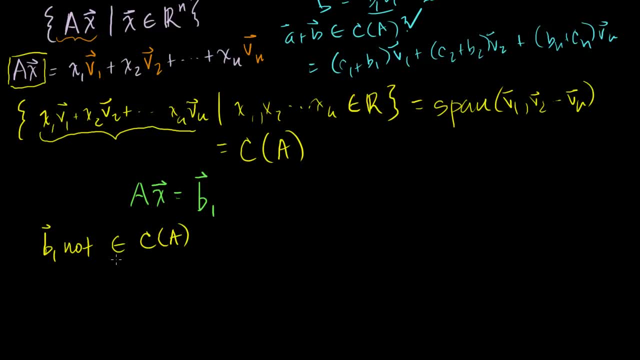 of the column space of A. Then what does that tell me? That tells me that this right here can never take on the value B1, because all of the values that this can take on is the column space of A. So if B1 is not in this, it means that this can. 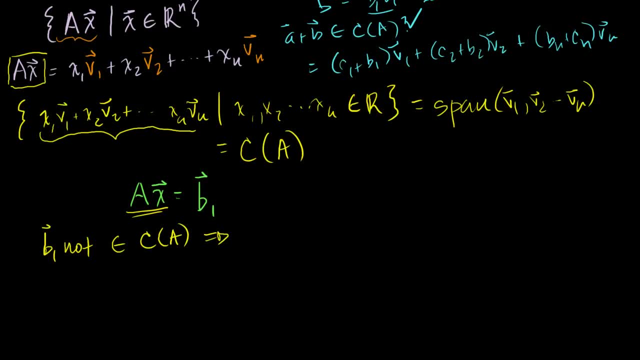 not take on the value of B1.. So this would imply that this equation we're trying to set up, Ax is equal to B1, has no solution. If it had a solution, if it had some solution. so let's say that Ax equals B2, has at least one solution. 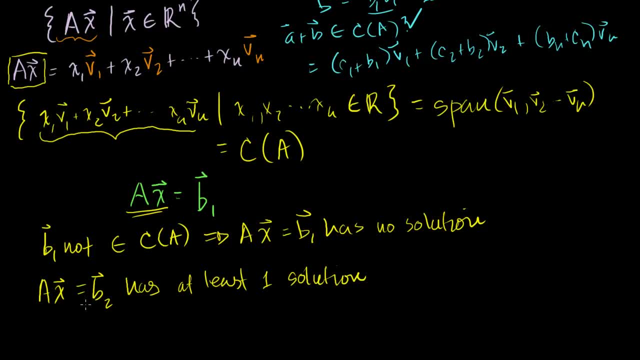 What does this mean? Well, that means that this for a particular x, or maybe for many different x's, you can definitely achieve this value Right, For there are some x's that, when you multiply it by A, you definitely are able to get this value. 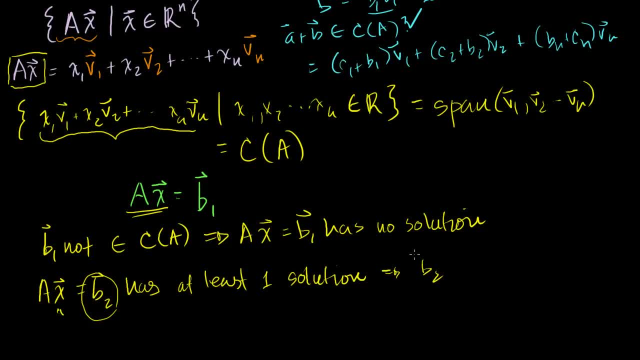 So this implies that B2 is definitely a member of the column space of A. Some of this stuff on some level, it's almost obvious. It comes out of the definition of the column space. The column space is all of the levels. 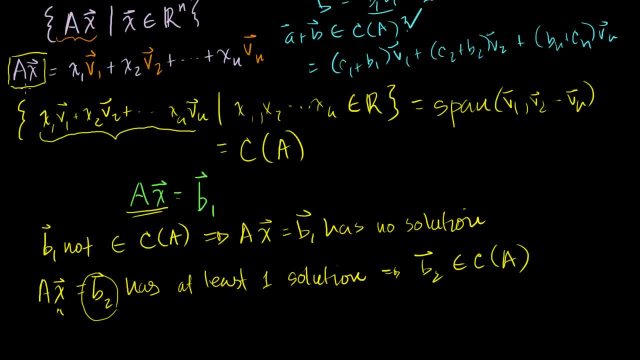 It's all of the levels Right, Right, It's all of the linear combinations of the column vectors, which another interpretation is all of the values that Ax can take on. So if I try to set Ax to some value that it can't take on,